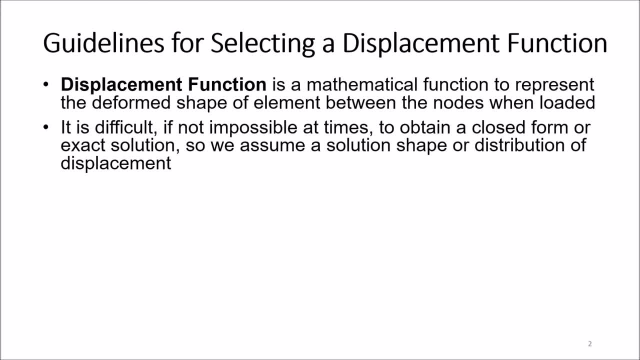 It is difficult or even sometimes impossible to obtain a closed form or an exact solution, So we assume a solution shape or a distribution of displacement using these displacement functions or approximate functions. The approximation functions should be: 1. Typically polynomial functions. 2. Continuous within the element. 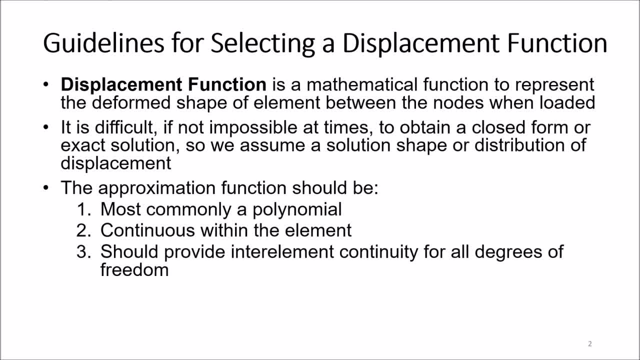 3. Provide inter-element continuity for all degrees of freedom, So within the element we have a continuous function for all degrees of freedom. And 4. It should allow for rigid body displacement and for a state of constant strain within the element. 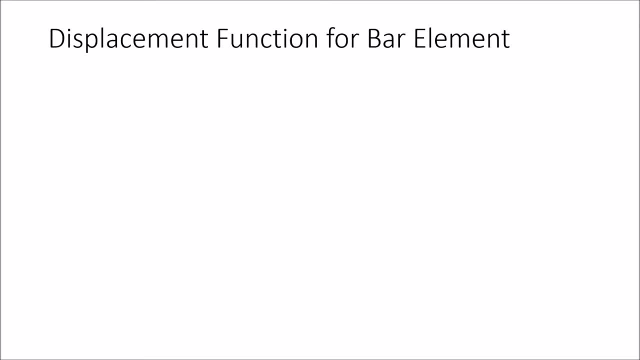 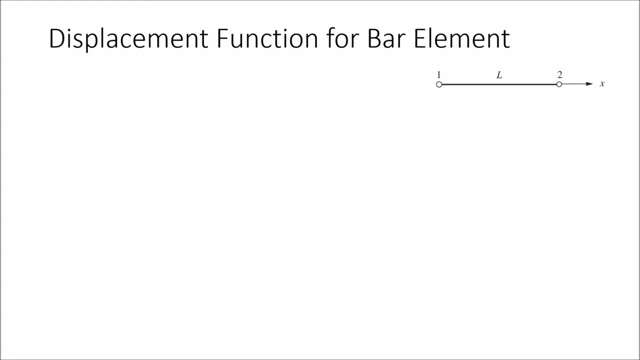 We are going to apply these guidelines to derive a displacement function for the bar element that we just developed, the stiffness matrix and so on element. so, as you can see, here we are looking at this bar element that has a start node 1 and an end node 2 and extends along the x-axis and has a 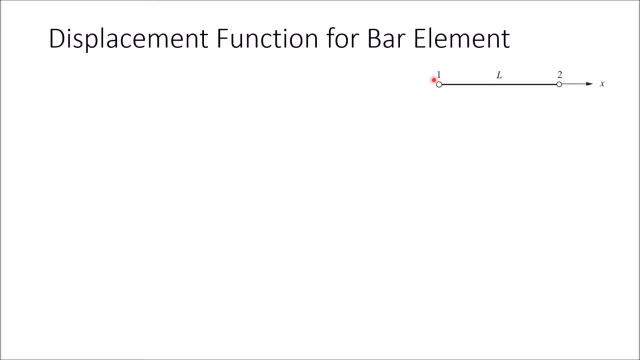 lengthurd now, where this bar with the two nodes has two degrees of freedom or two nodal displacements. two nodal displacements, namely we have here a u1 and we have here a u2, so at each node we only have one nodal sprints. so 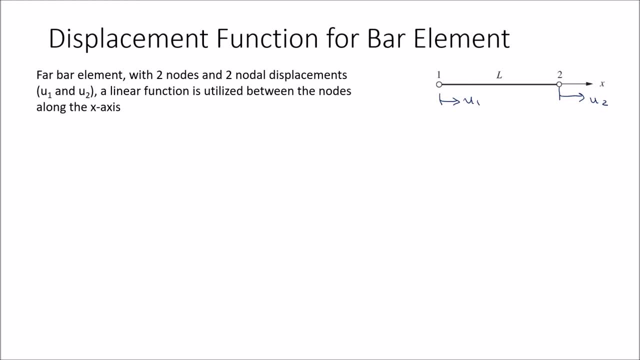 displacement. When we look at a displacement function to describe the displacements between node 1 and node 2, so we know the displacement at 1,, we know the displacement at 2, but we are in need of a shape function or an approximate function to give us the displacement throughout. 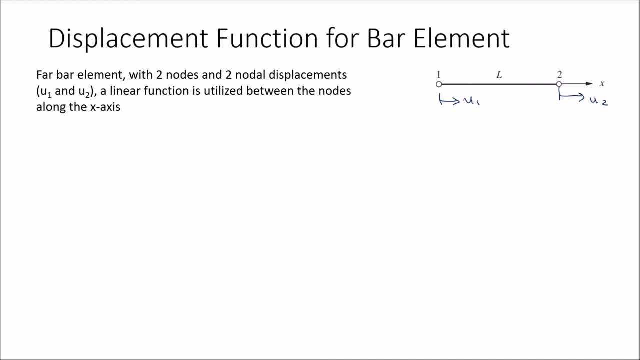 the element. The polynomial that we're going to use here would be a linear function between the nodes along the x-axis. So this linear function is going to look something like this: At node 1,, we know that the displacement is u1, and at node 2, the displacement is u2.. If I connect, 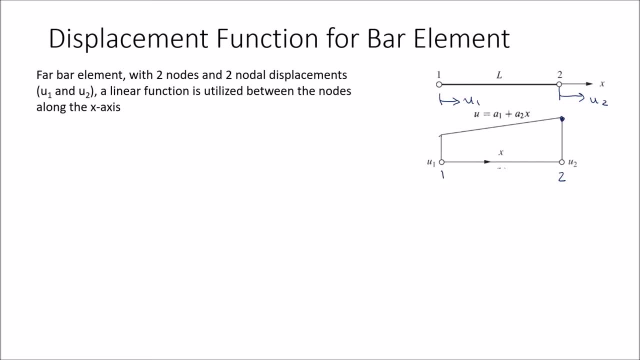 these two displacements by a straight line. this straight line has a linear relation and u at any distance. x along the element or within the element may be described by: u equals to a1 plus a2, x. I may also write this equation in matrix form as: u equals to. 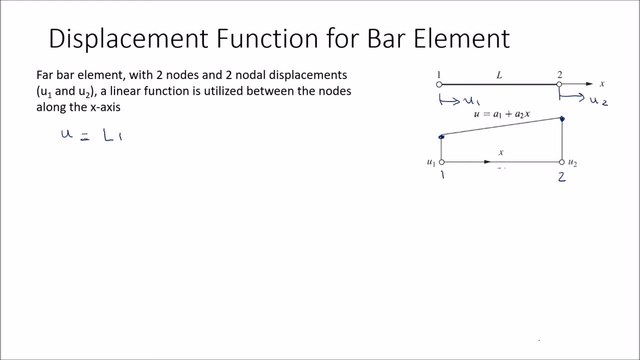 1 and x a row 1 and x a row 1 and x a row matrix multiplied by a column matrix: a1 and a2.. So this is the same as saying a1 plus a2 times x. Now we should be able to solve for these coefficients a1 and a2, and please note that. 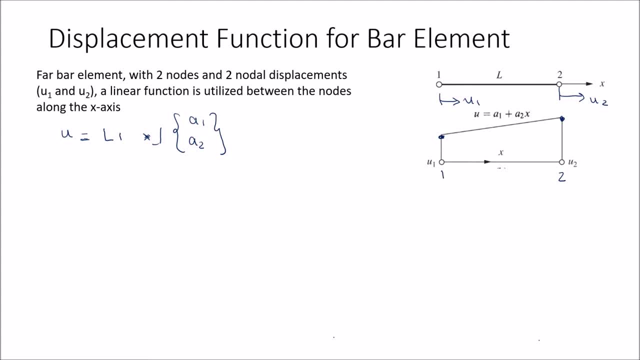 a linear function serves well here, because the number of coefficients is the same as the number of coefficients ля proposal, trials of degrees of freedom. we have to know the displacements and we have two unknown coefficients, a1 and aç. so using boundary kernel, boundary conditions, we should be able to solve for these coefficients. 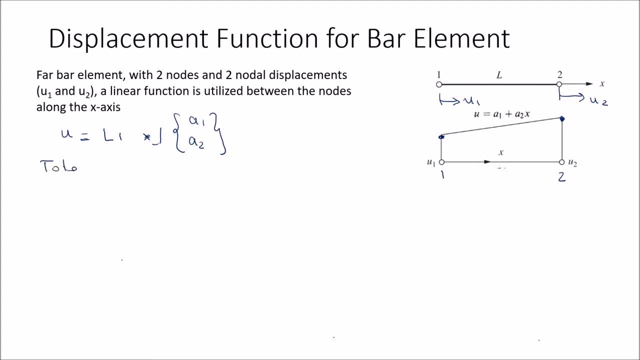 So I can say here that the total number of coefficients which we have added is equal to sorry $8,.50,. so this is nothing in addition to our number of coefficients. Moving on y reading here, we should do a Basically for each of these coefficients. 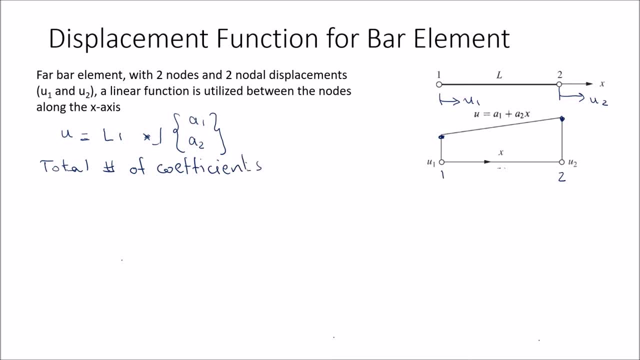 remember that we should have número of coefficients and number of degrees of freedom. we have two nodal displacements and we have two unknown coefficients, a1 an a2. using boundary conditions, we should be able to solve개 equal to the total number of degrees of freedom, and for this element, this is 2. 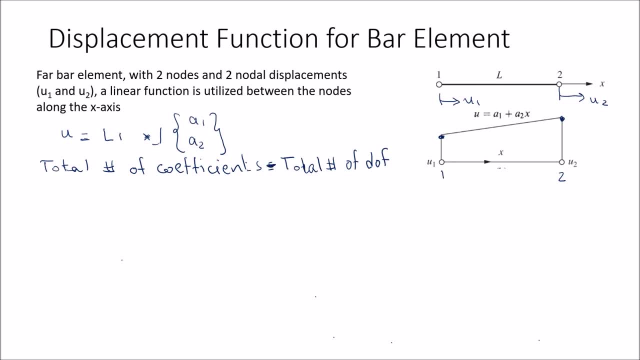 now, in order to evaluate these coefficients, we are gonna use the boundary conditions. so I can come here and say: at X equals to 0, this is at node 1. so at X equal 0, we have u equals to u1. if I use my equation and substitute: 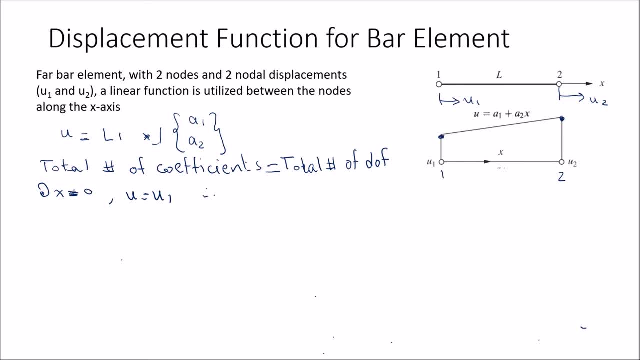 for X equals 0, I can conclude that u1 must be equal to A1 or A1 equals 0 to u1. so here i solved for the first coefficients. next, at x equals to l, u is equal to u2. therefore u2 is equal to u1 because a1 is equal to u1 plus a2. 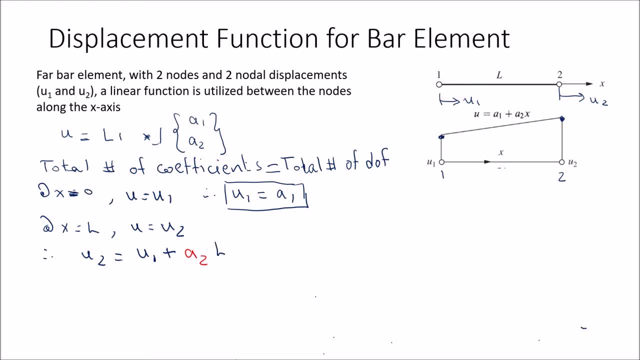 multiplied by l. so we can solve for a2, and a2 would then be equal to u2 minus u1 over l. so now we're, having solved for the two coefficients, we can write that u is equal to u1 plus u2, minus u1 over l multiplied by x. 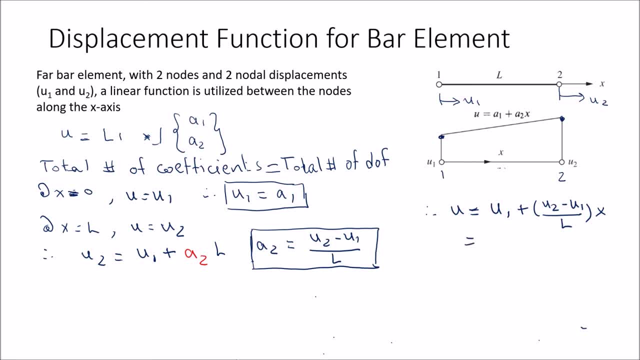 which is, uh, maybe expressed as u1 plus u2 over l times x minus u1 over l times x. i can write this as equal to 1 minus x over l times u1 plus x over l times u2. in matrix form, i can write it as u equals to: 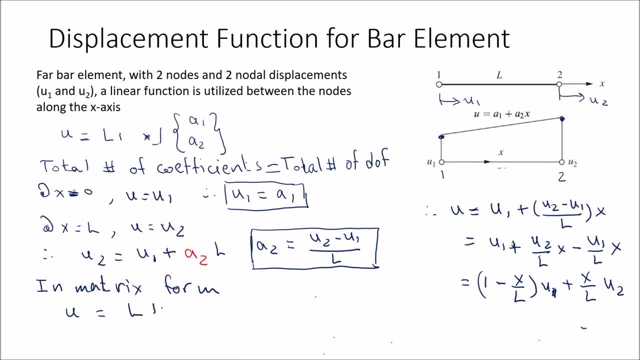 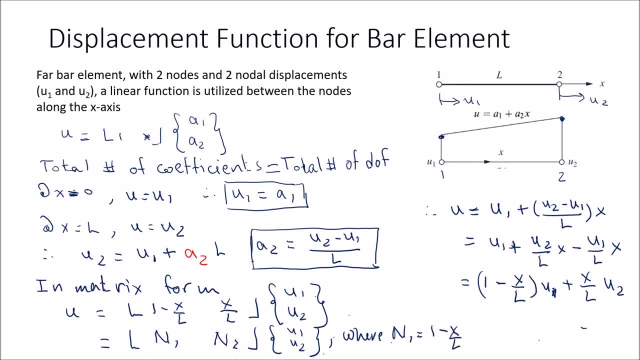 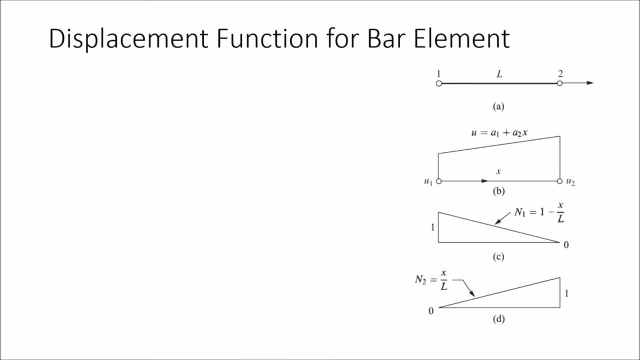 X over L and n2 is equal to X over L. n1 and n2 are shape functions corresponding to the degrees of freedom or the nodal displacements u1 and u2. so, just to remind you, were able to express u as equal to n1 and n2 multiplied by u1 and. 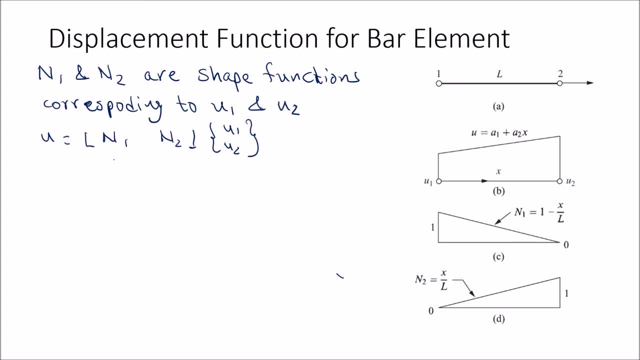 u2. if I plot n1 along the x-axis, you will notice that n1 was 1 minus X over L, 1 minus X over L. so here I'm looking at n1 and n1. if you substitute X, equal 0 would have a value. 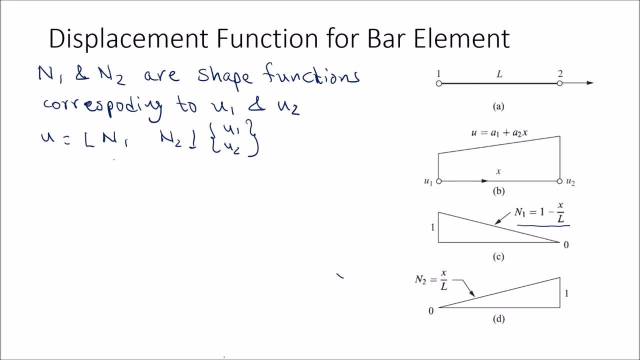 of 1 at X equal 0 or corresponding to node 1. it's called n1, corresponding to degree of freedom, 1. so we have a value of unity at X equal 0 at node 1 and would value of 0 at node 2. if I plot n 2, which is equal to X over L, you will notice. 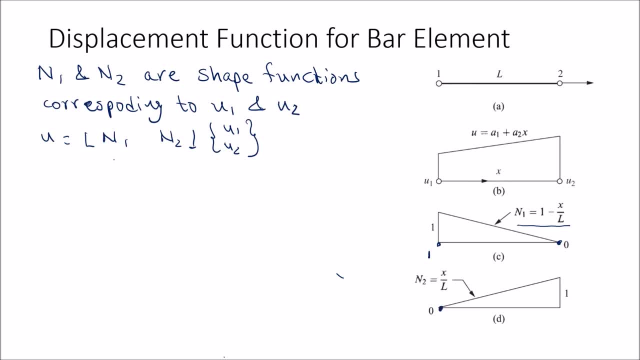 that n? 2 is equal to 0 at node 1 and equal to unity at node 2 at node 2. from this we may conclude that the shape functions n? i's are shape functions and n? i's for any degree of freedom. express the. 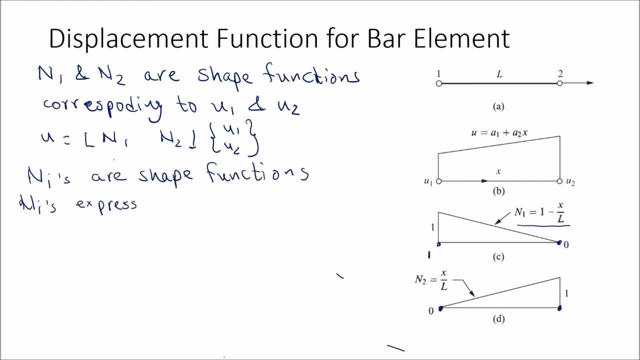 the shape of assumed displacement function over the domain with the i'th element, one, the two, the two, the other, the, the, the and S. We can also show that n1 plus n2 at any given x along the element is equal to 1.. So if you look at, x equals 0, we have 1 plus 0 is 1.. 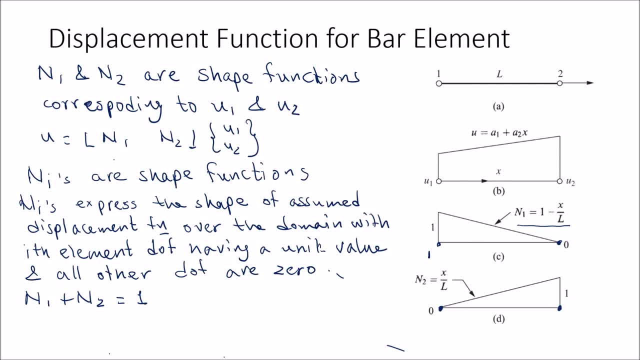 At x equals l, I have a 0 plus 1, which is 1.. If you go anywhere at the same x and you add this n1 to this n2, the summation is going to be equal to 1.. So n1 plus n2 is equal to 1 for any x value.